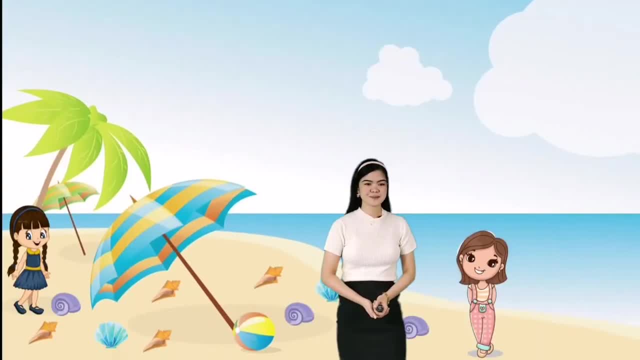 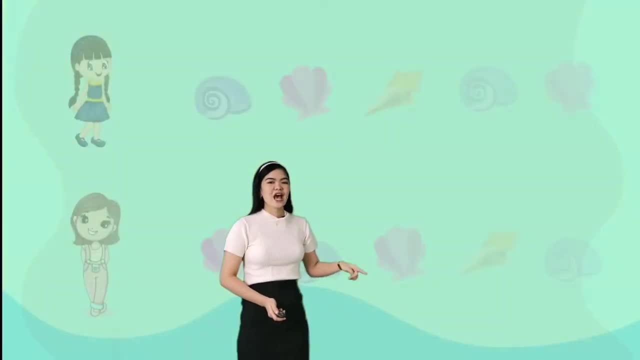 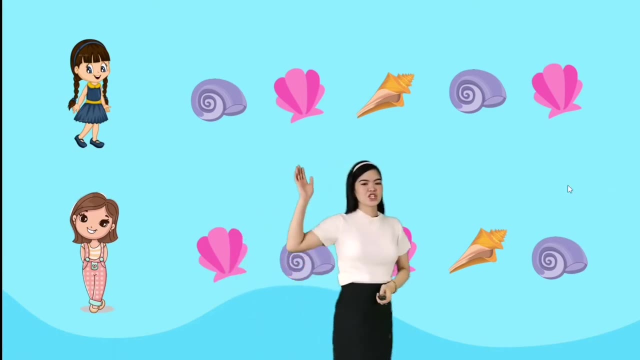 First the equal symbol. Janice and Siti are picking seashells at the beach. How many seashells does each girl have? First, let's begin with Janice. So Janice have 1,, 2,, 3,, 4, and 5.. 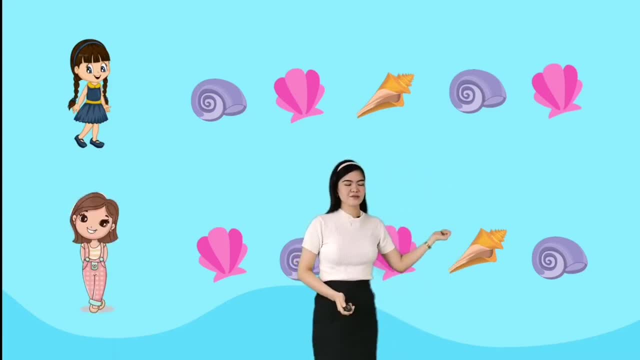 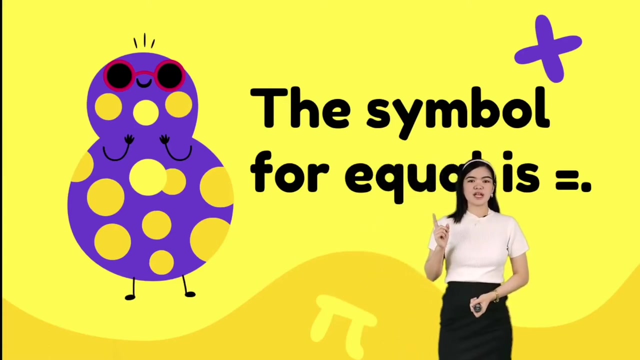 How about Siti? Siti have 1,, 2,, 3,, 4, and 5.. They have an equal number of seashells. So what is the symbol for equal? The equal symbol is written as, So we can write: 5 is equal to 5.. 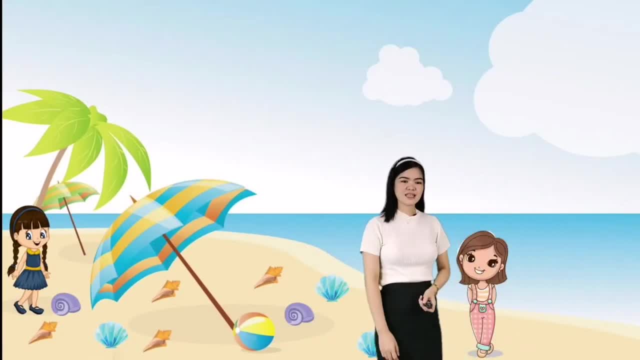 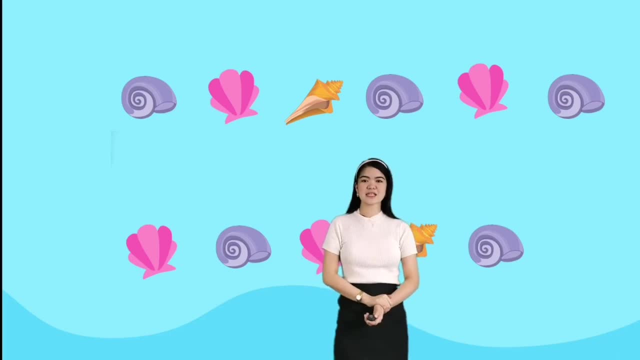 On the next day, Janice and Siti collect the seashells again. So let's take a look how many seashells they got. So Janice got 1,, 2,, 3,, 4,, 5, and 6.. 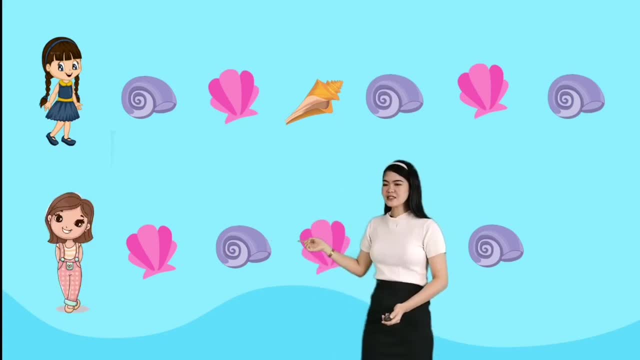 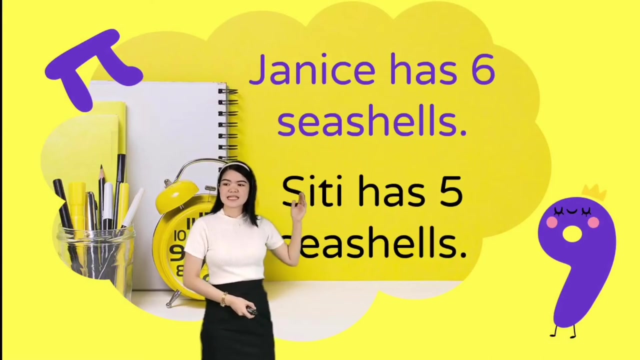 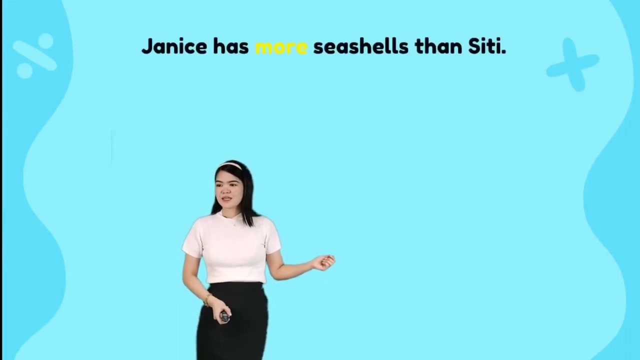 How about Siti? Siti got 1,, 2,, 3,, 4, and 5.. So therefore we conclude that Janice has 6 seashells and Siti has 5 seashells. Janice has more seashells than Siti, so 6 is more than 5.. 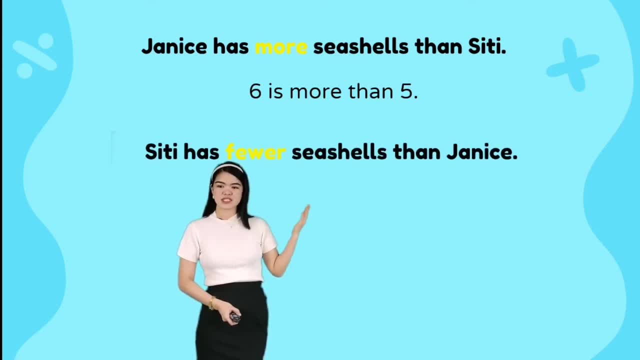 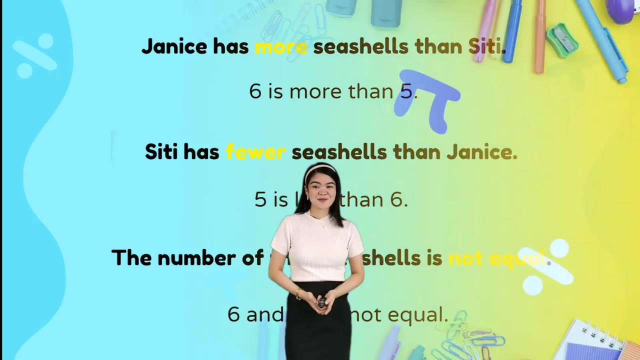 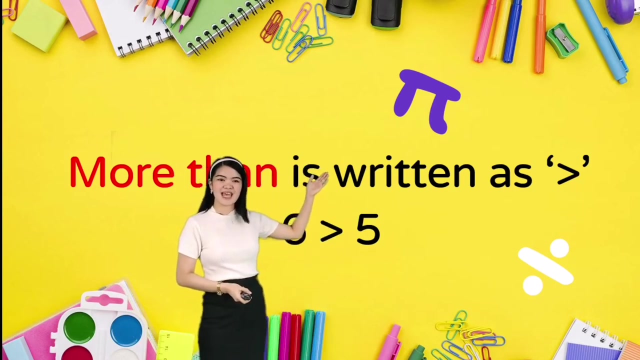 While Siti has fewer seashells than Janice, so 5 is less than 6.. The number of their seashells is not equal, So 5 and 6 are not equal. Let's have another example: More than is written as the greater than symbol. 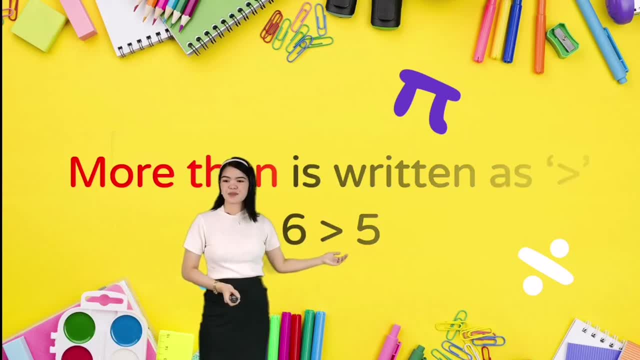 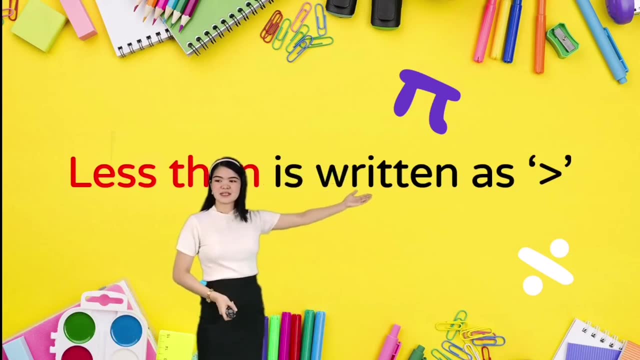 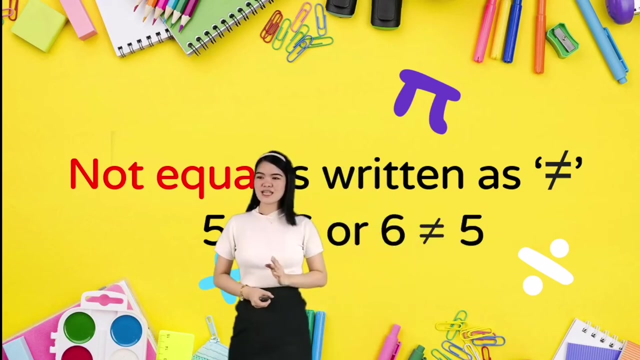 So 6 is greater than 5.. Less than is written as less than symbol, So 5 is less than 6.. Not equal is written as this one, So 5 is not equal to 6, or 6 is not equal to 5.. 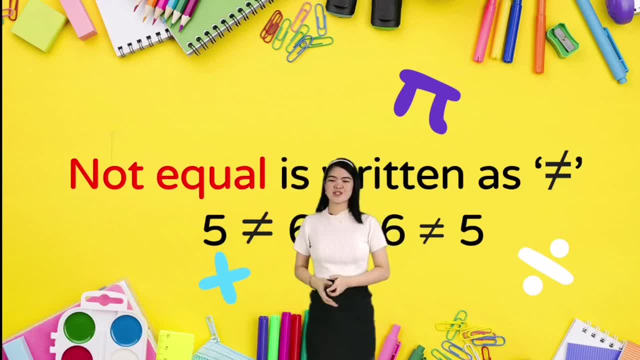 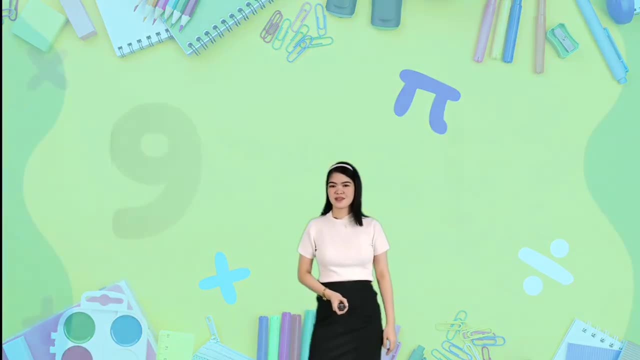 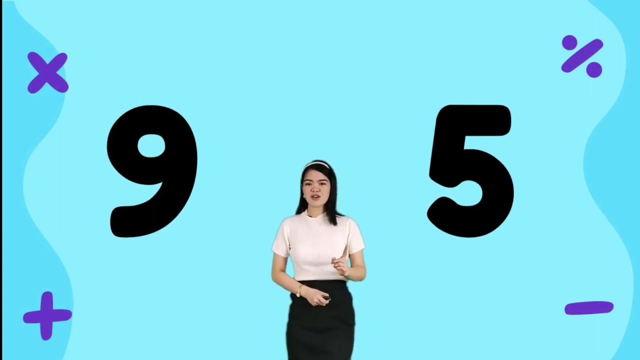 Once again, not equal is written as this symbol. So 5 is not equal to 6, or 6 is not equal to 5.. Let's have another example. We can use the mouth of an alligator to represent its symbol. 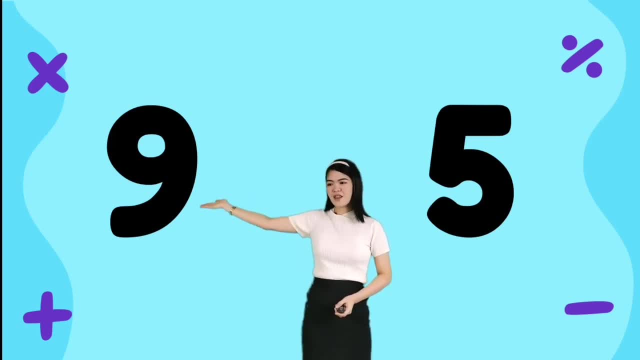 So we have here 9 and 5. Which one has a larger number? 9 is larger than 5.. So the alligator's mouth is open to number 9.. And we can say that 9 is greater than 5.. 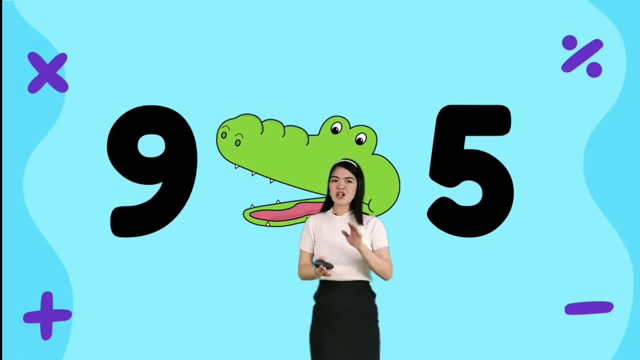 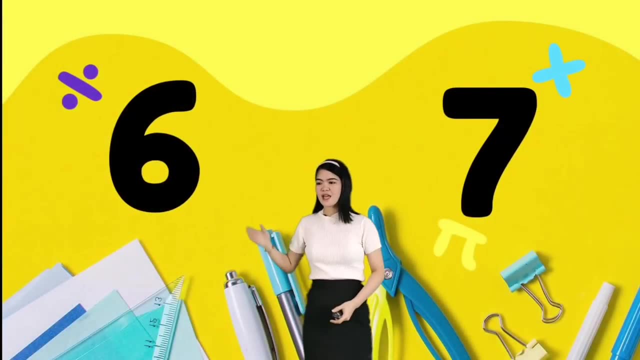 Always remember that his mouth is always open to the larger number. Next one: we have 6 and 7.. Which one has a larger number? 7 is the larger number. Which one has a larger number? So this one is the larger number. 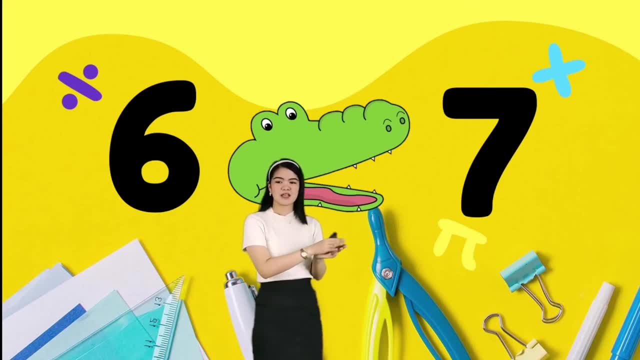 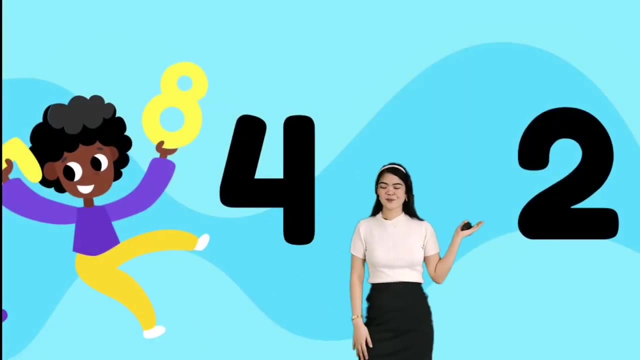 So the alligator's mouth will open to number seven. Six is less than to number seven, Six less than seven. Next, we have four and two, Which one has a larger number Four, Very good. So the alligator's mouth will open to number four. 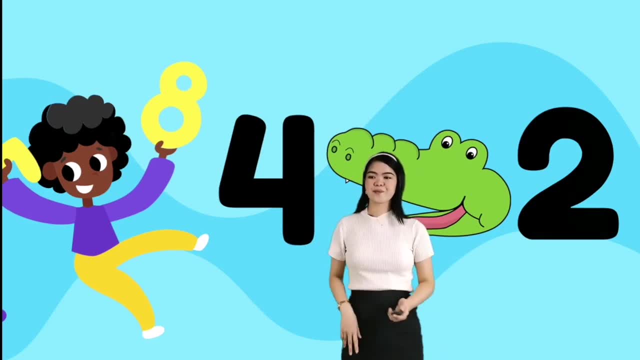 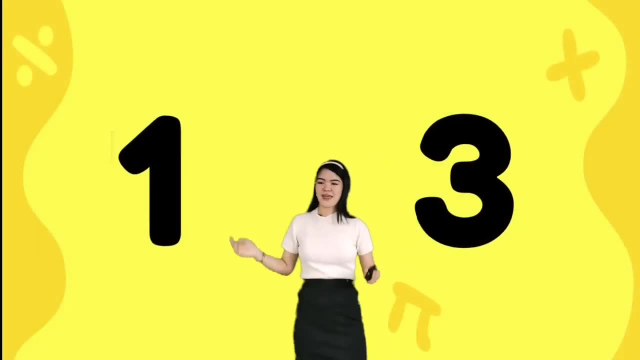 Four is greater than two. Another example is one and three. Which one is the larger number? Number three. So the alligator's mouth will open to number three. So one is less than three. Next we have our activity. Please get your book.